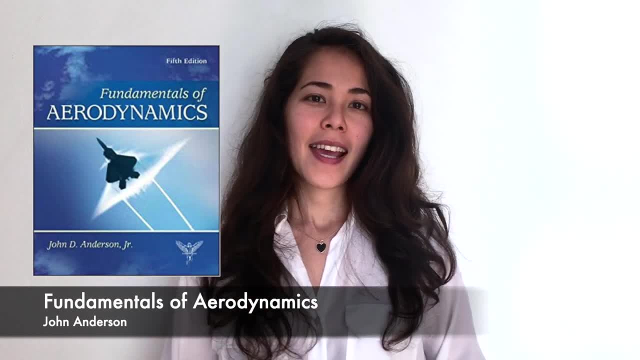 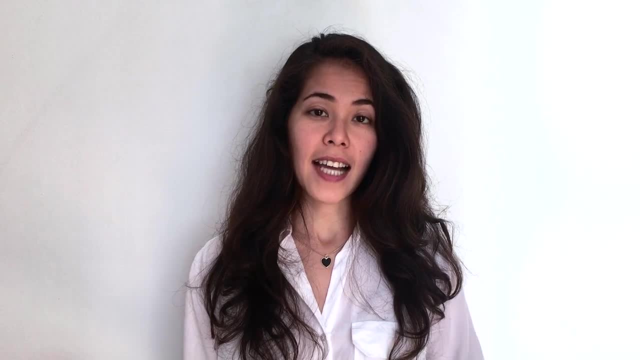 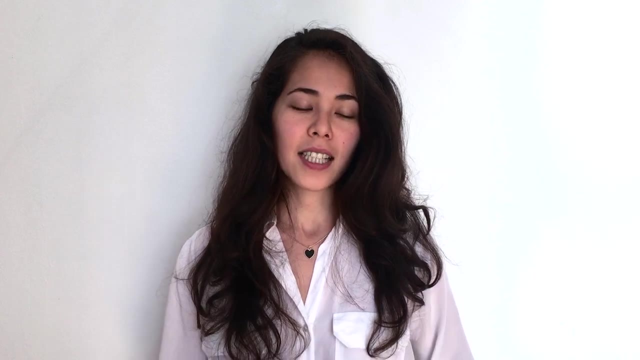 Anderson. It's a pretty thick textbook and I think I used it in my third year for incompressible flow class, So this textbook is kind of considered a classic in the aerospace engineering community and you can learn about aerodynamics from this textbook, obviously. but the level of content is pretty difficult. 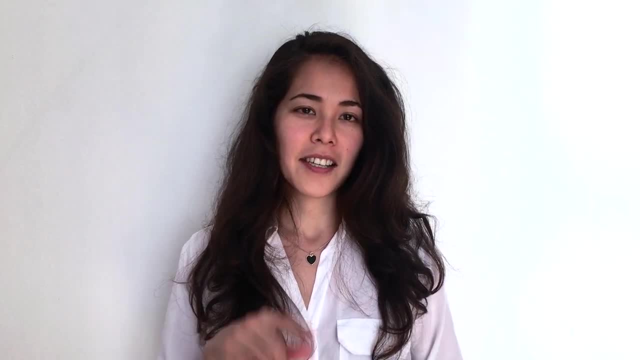 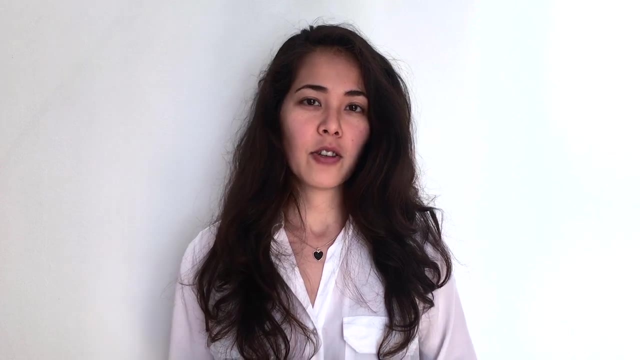 because I really don't have a lot of experience in aerodynamics so I can't really explain it to you, But I think it's a really good textbook because I remember it was difficult for me to understand the capital gamma sinks and stuff like that. I still remember reading about those things, but I cannot. 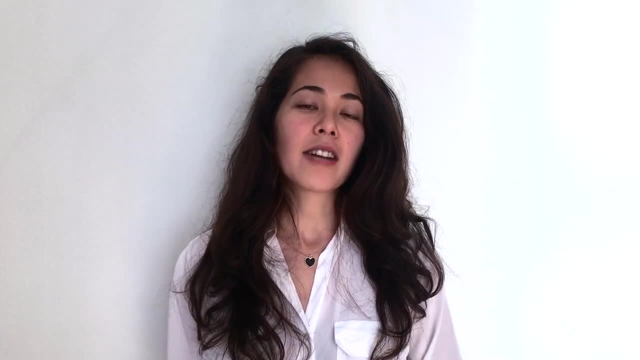 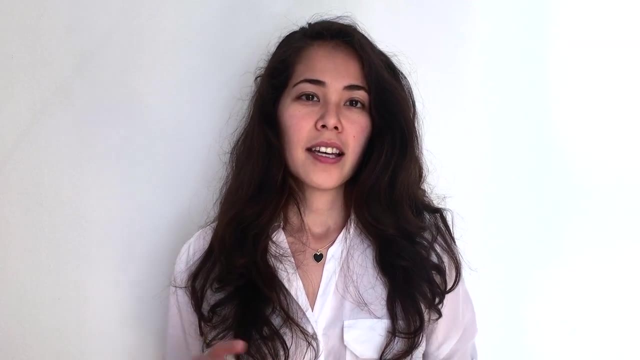 tell you right now exactly what it was, And let me tell you that I read one page maybe 50 times to try to understand it. But don't get scared by that, because if you're really into aerodynamics, this textbook gives you a very solid basic. 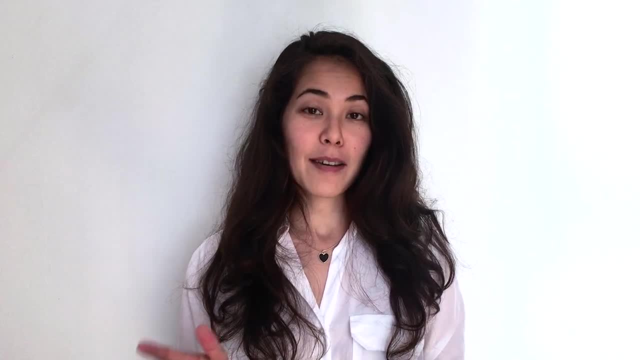 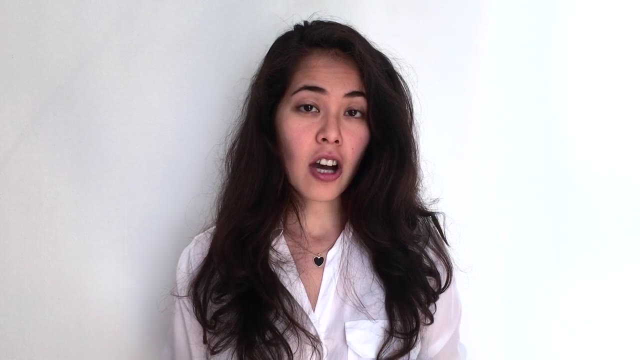 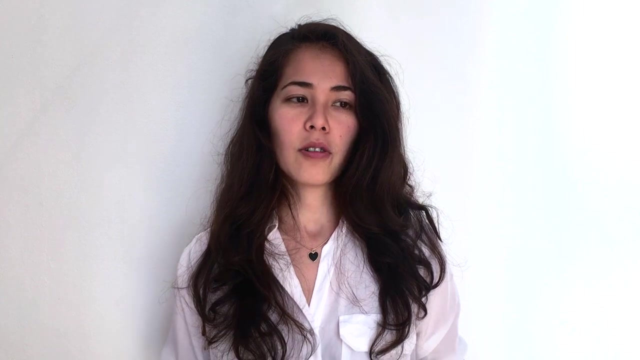 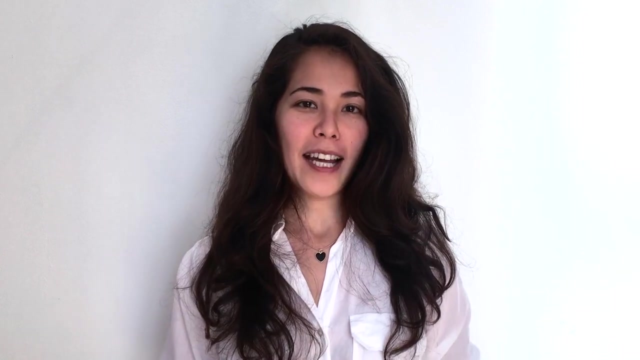 knowledge about aerodynamics. And one more thing about American textbooks is that they are freaking expensive, Expensive. The average cost of one textbook is about 80 to 120 dollars. Some textbooks cost even more, maybe 150 dollars. So at the end of this video I will teach you a few life hacks to try. 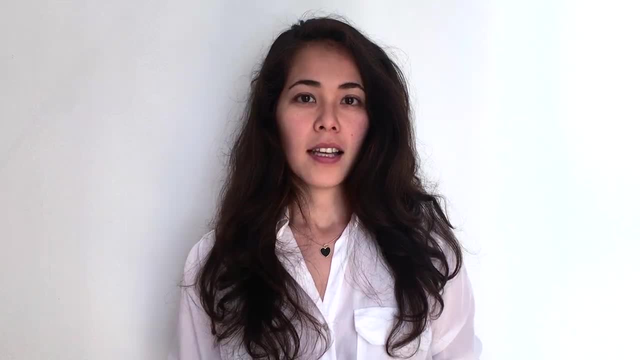 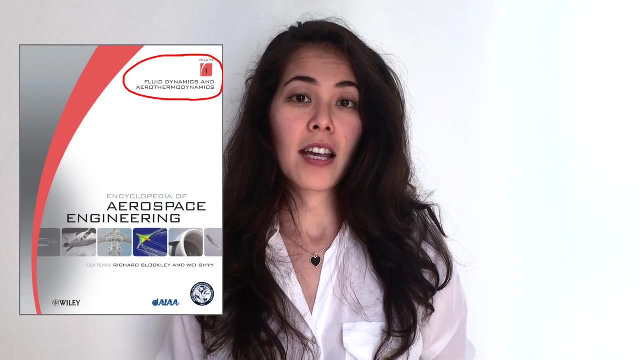 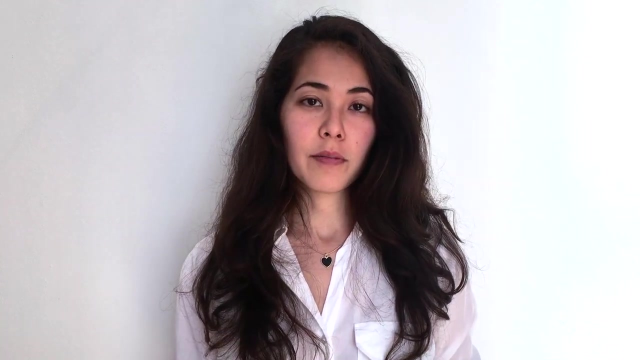 to save some money instead of buying those textbooks, And if you're curious about the cost of the textbooks, I will also give you a link to the video where I get content for my videos. This was from the Encyclopedia of Aerospace Engineering that I found in a library at the university where I worked, And I will put. 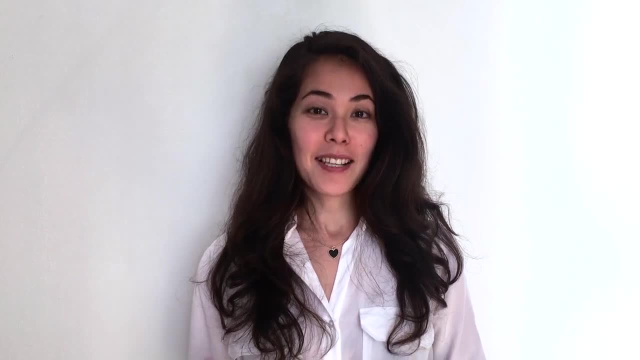 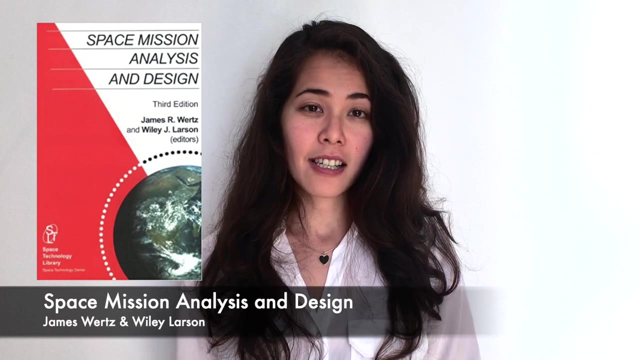 a link to it below and also you will be able to see it right now on the screen. Okay, let's move on to the second textbook which I still remember, And I remember the cover And I use it in my senior year for senior design class In my program at the University of 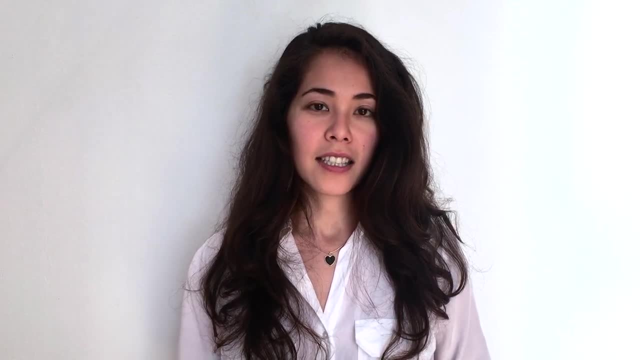 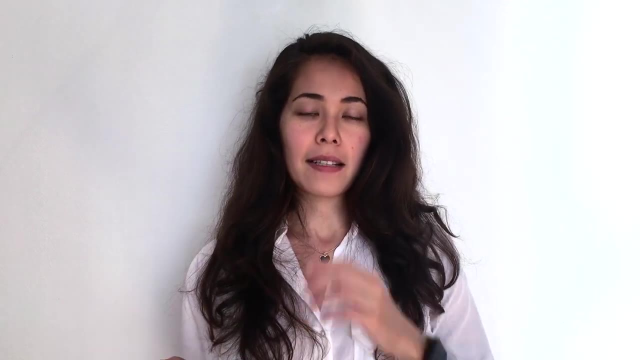 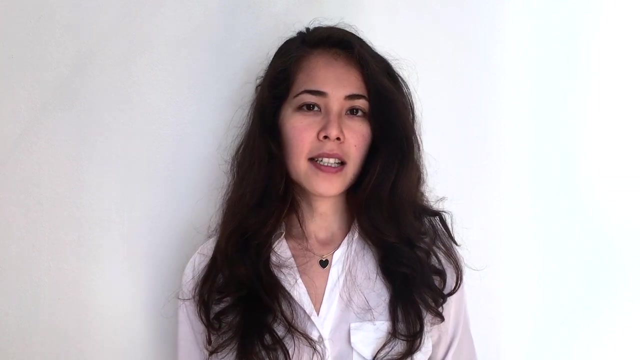 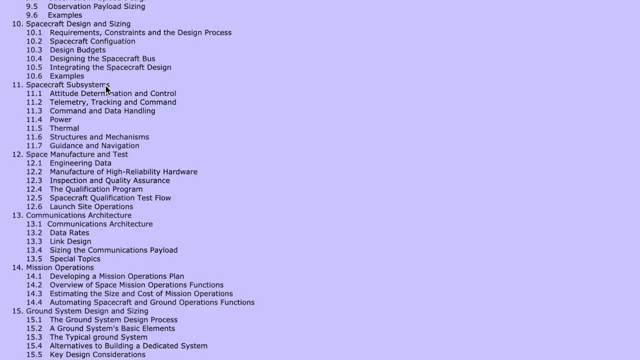 Illinois, at Urbana-Champaign. in your senior year you could choose your direction, what you wanted to do- Either Aeron or space. So I chose space and we were divided into teams in our class to prepare designs of a project. So we use this textbook to divide our team into sub systems, for example, electrical. 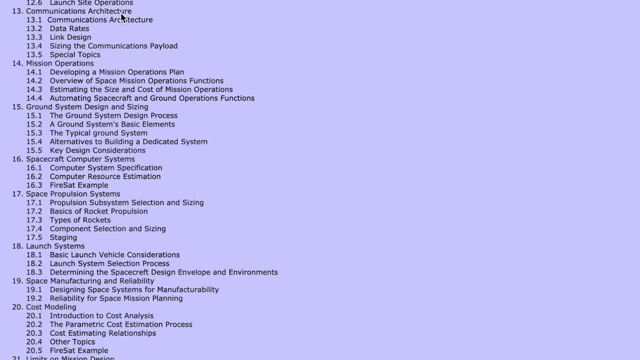 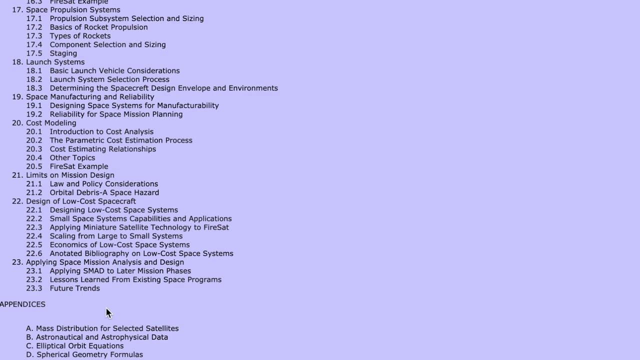 or power and data handling and stuff like that. So if you open this textbook, you will see that it's divided into many subtopics or subsystems of designing a huge aerospace system. So if you want to work in aerospace systems design in the future, 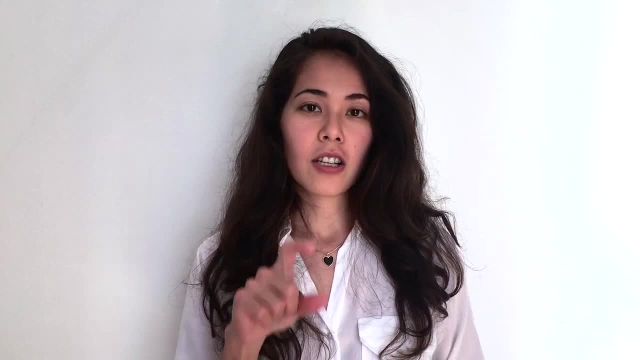 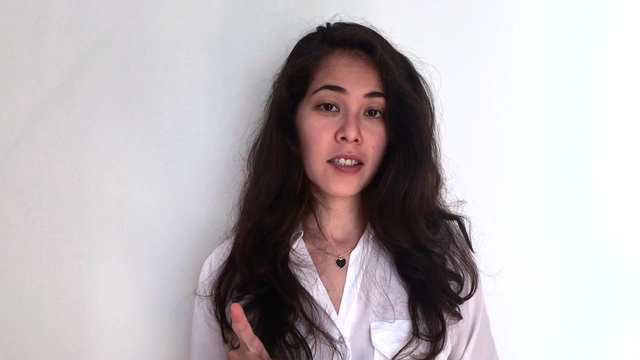 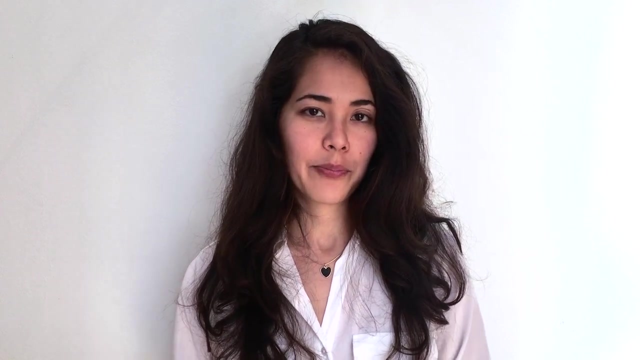 this textbook can give you knowledge in about all of the subsystems of a huge aerospace system. But this textbook is written much easier compared to the fundamentals of aerodynamics, But it has a lot of data which is difficult to remember. So if you read a textbook like that which is complicated, always have a 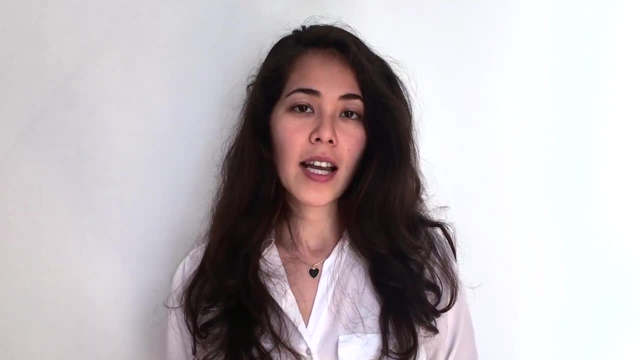 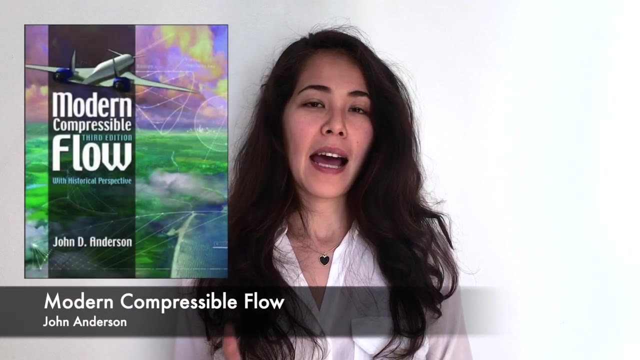 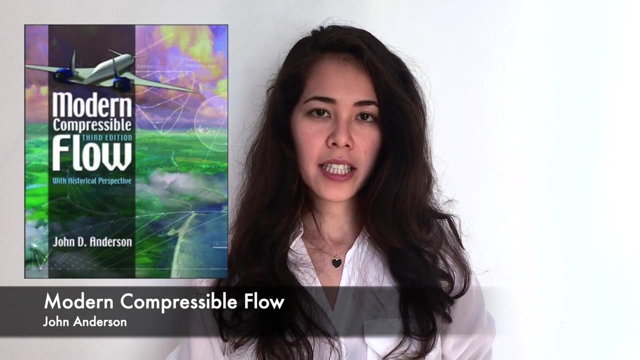 piece of paper or notebook next to you where you can write down some important facts. Alright, the next textbook. I don't remember how it looked, but we used it in our compressible form And I'll show you the cover of the book on the screen. So this textbook talks about. 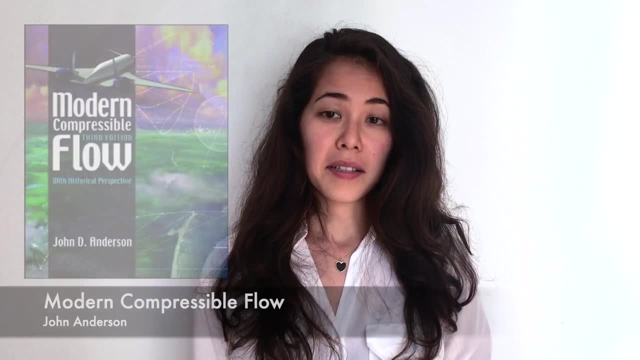 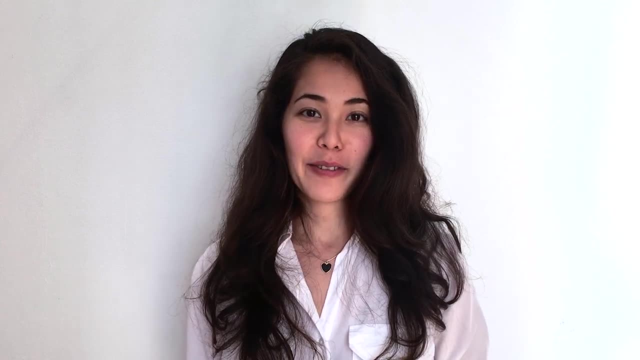 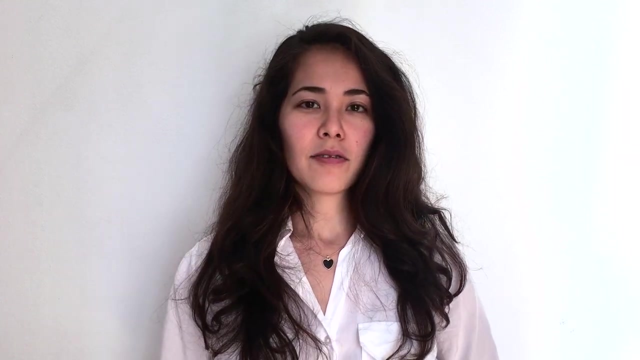 the compressible flow and propulsion. I still remember my professor, who was very nice and if you studied hard he always gave you good grades. Alright, that's completely irrelevant for this video, But I remember I was trying my best in that class and it was pretty interesting because we learned about shockwaves. 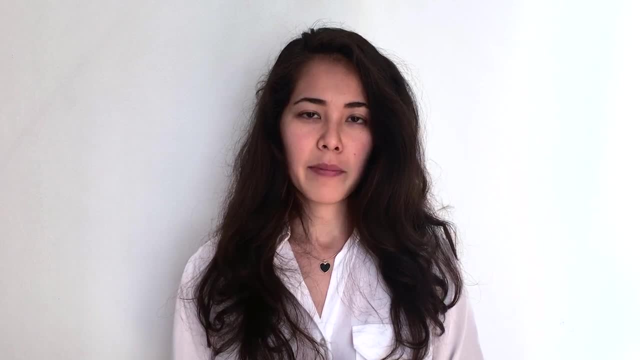 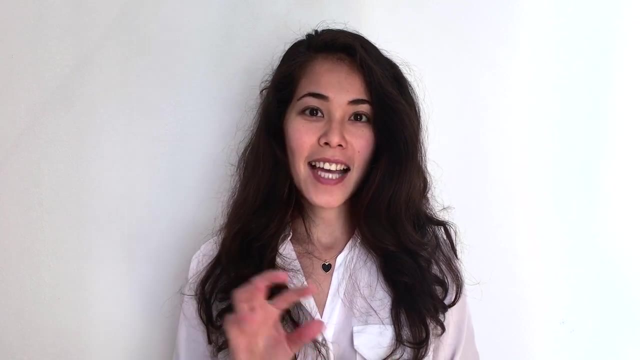 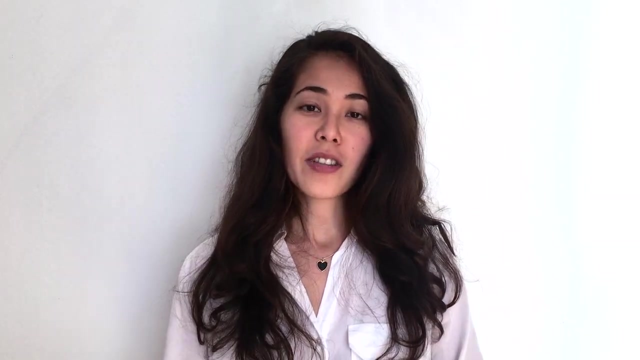 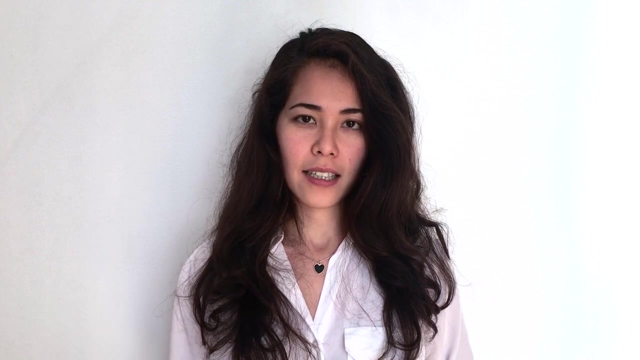 earthquakes, the speeds higher than Mach 1, we learned about choking the flow. and for propulsion we learned about turbojets, ramjets, and we learned how to calculate all those parts to get the thrust for the engine. So the textbook was well written and it was pretty interesting and it's easy to understand it. So I 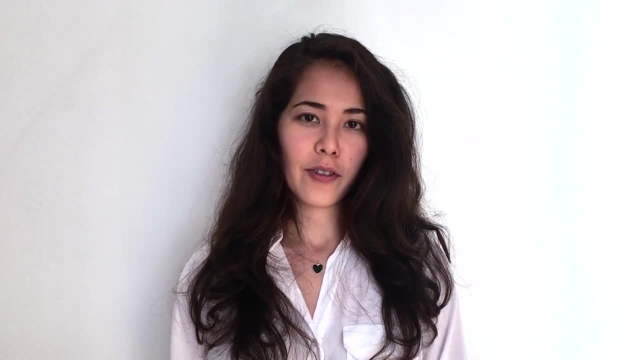 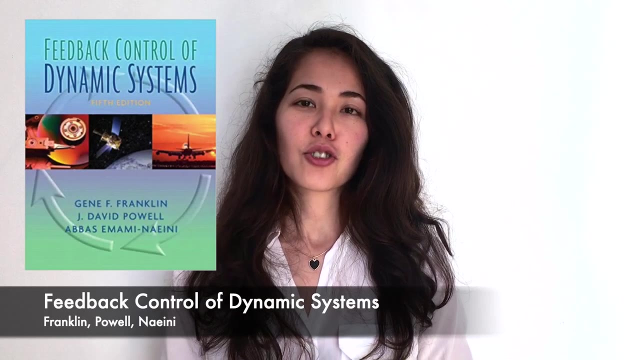 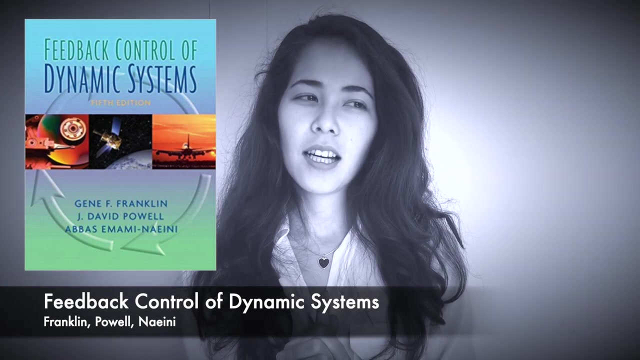 highly recommend it if you're interested in compressible flow and air flow speeds higher than Mach 1.. Alright, next textbook was for my control systems class, or it was called feedback control. it was called feedback and control systems, No, something like that. Okay, control and. 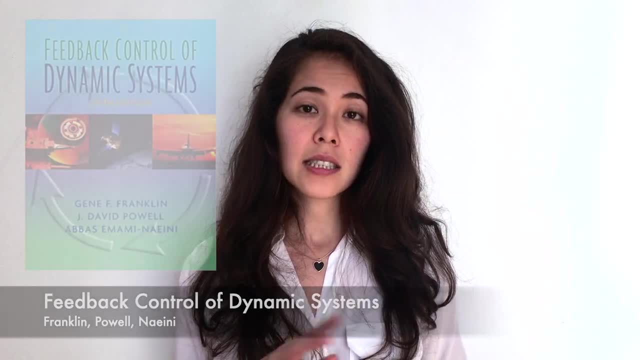 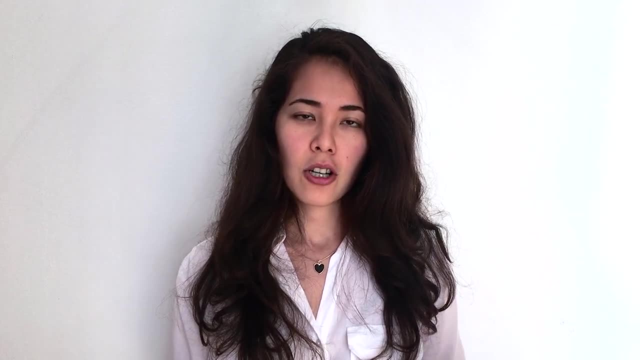 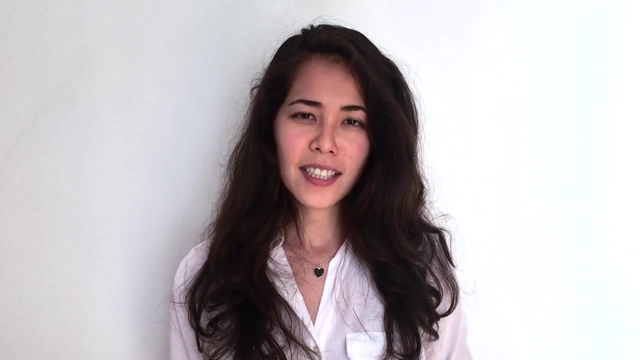 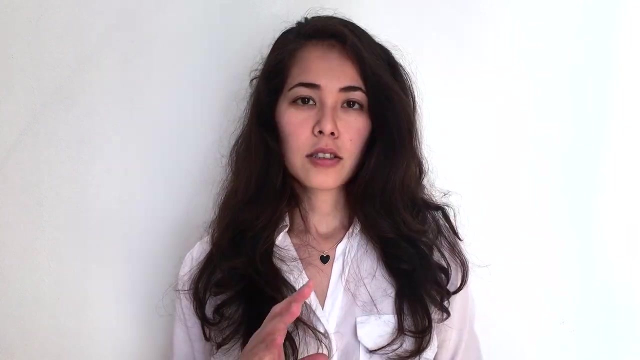 feedback systems. So basically it was a class about control systems and control loops, feedback loops. So I was a teaching assistant in this class before, So now I understand this topic better, but at that time in my junior or senior year I did not know anything about it and the textbook was terrible. So instead, 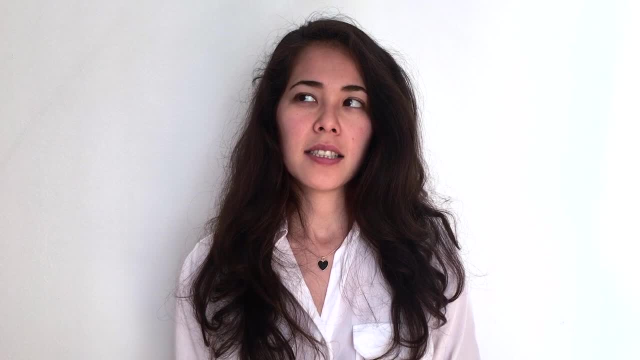 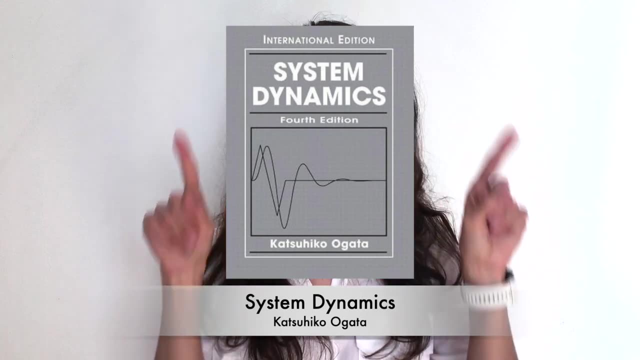 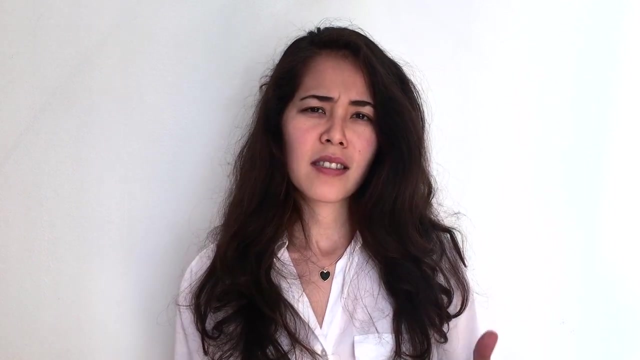 of reading this textbook, that we had read a different textbook by Japanese author. I can't remember his last name, but it's gonna be here on the screen. When I was a teaching assistant for linear control systems, I read the textbook, or I used this textbook as a reference, and it's much better written. 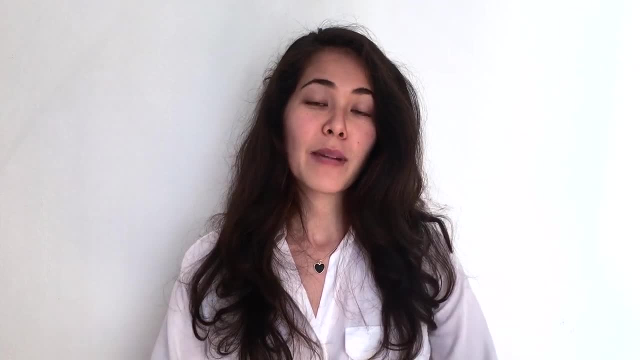 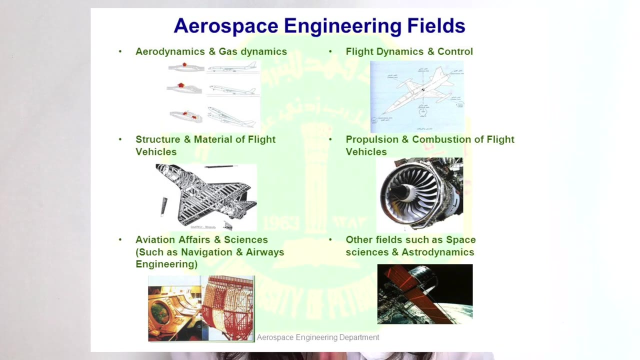 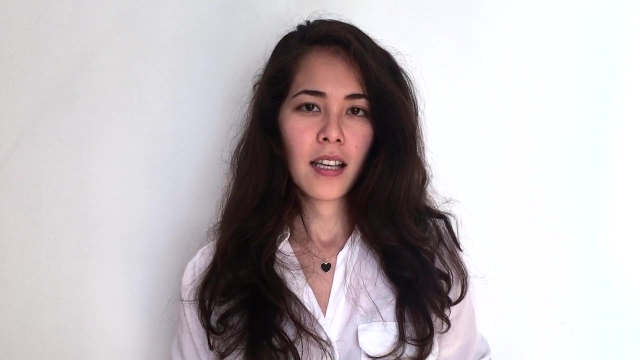 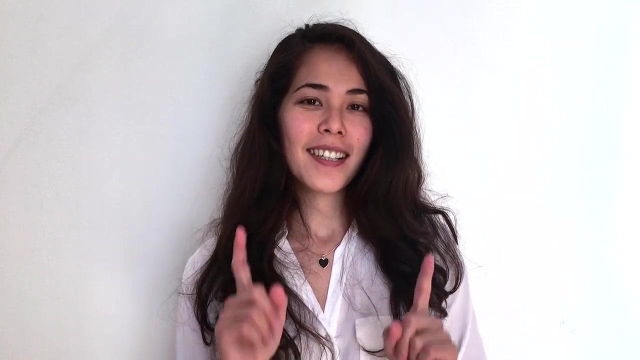 and better explained. So remember, in my very first video I explained how aerospace engineering is divided into many subfields and if you are into controls or control systems, then you need to be very fluent with feedback loops, Kalman filters and stuff like that. Okay, next textbook is a. 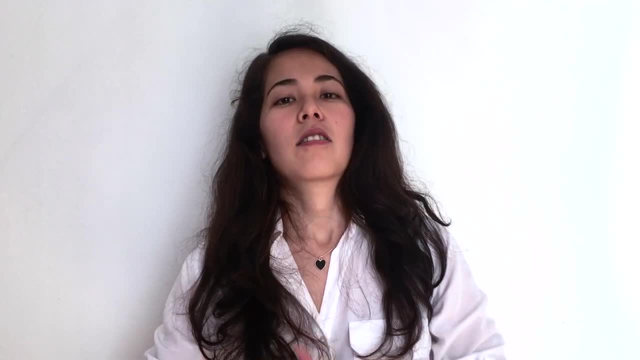 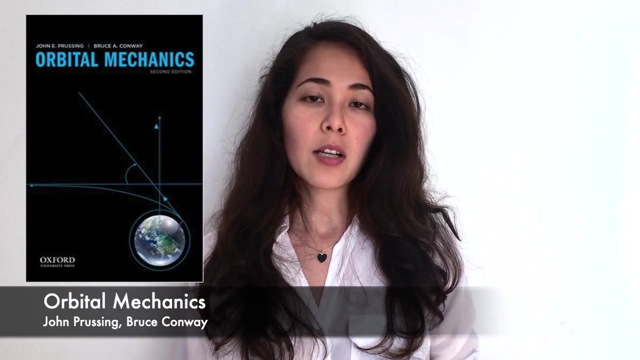 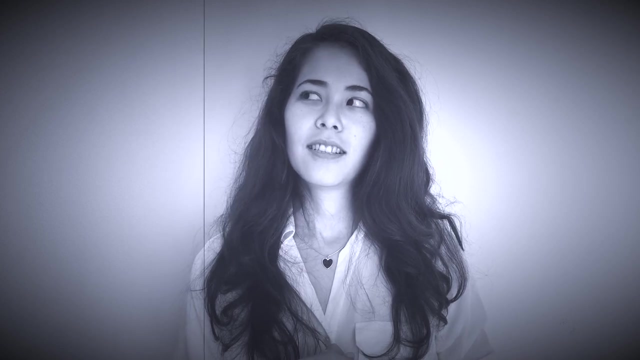 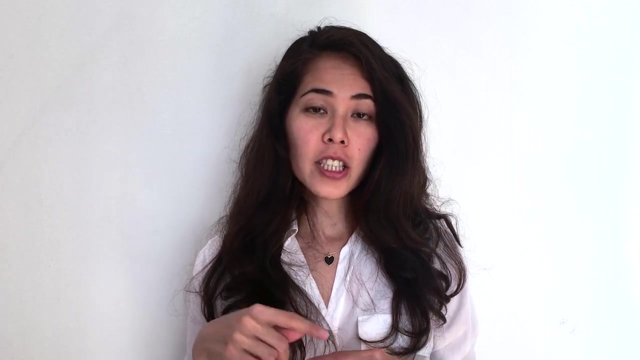 also very good. It's orbital mechanics. So from this textbook you can learn about orbital mechanics, obviously. but what does that include? It includes changing the orbits using a- what's his name? Using a Hohmann transfer and calculating how much fuel you need for some type of transfer. how much fuel you need to change. 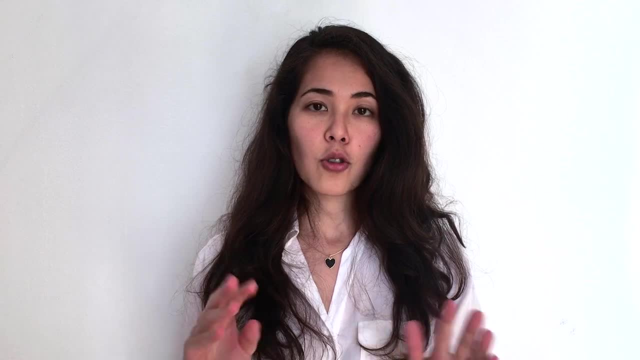 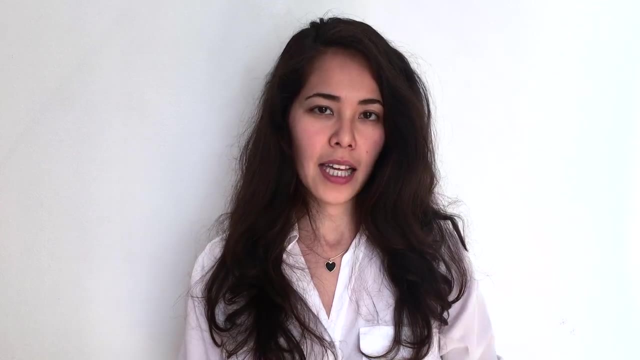 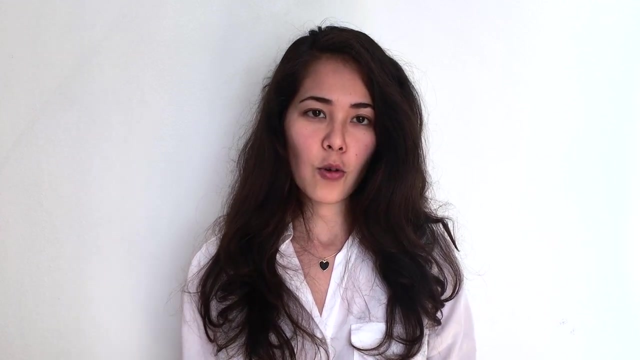 the inclination of the orbit and also what are the velocities that you deal with, how much velocity you need to change the orbit and stuff like that. So I think, because I'm more interested in space, this class was very interesting and this textbook was useful, So I highly recommend it. Alright, two more classes. 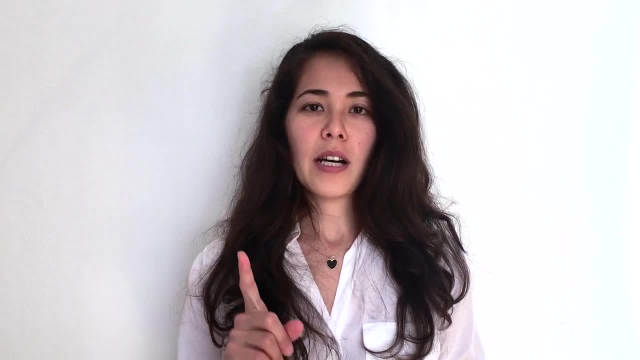 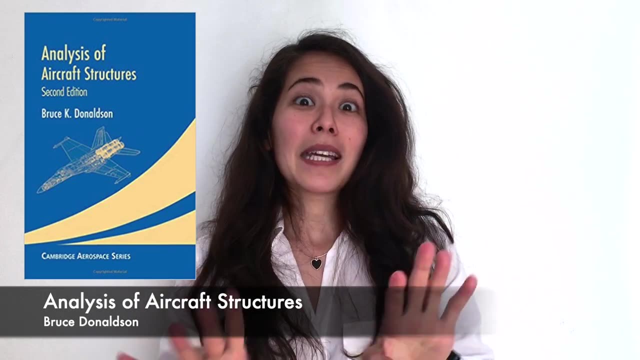 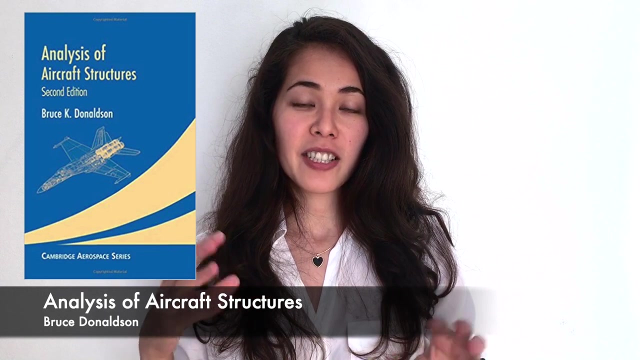 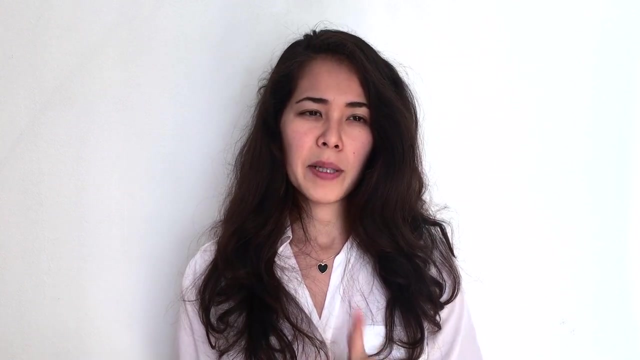 two more textbooks that I recommend: One about structures, which is definitely not a topic of interest, but maybe it's yours. So in structures you deal with a lot of bending moments about the materials that are used in aerospace, and I wouldn't say it's easily written, because I also remember reading one page. 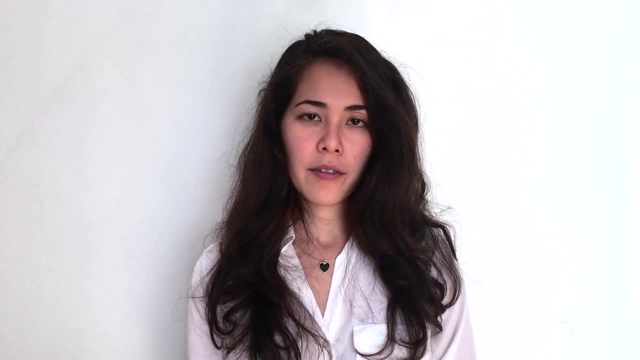 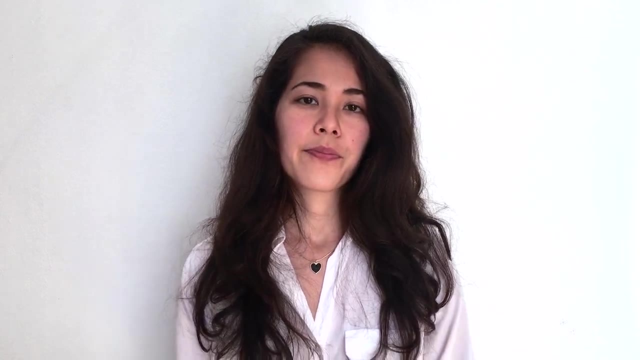 many, many times, but in the end it was useful to prepare for the exam And you can learn a lot about structures from this textbook. It's a very comprehensive textbook. The final textbook that I want to share is Electric Propulsion, and I remember I 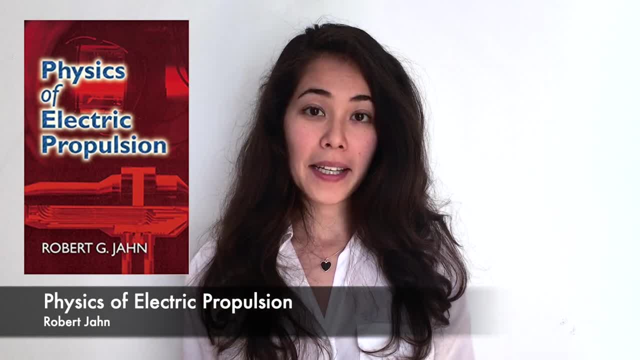 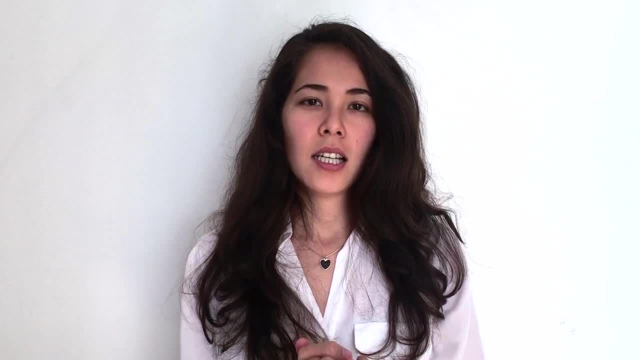 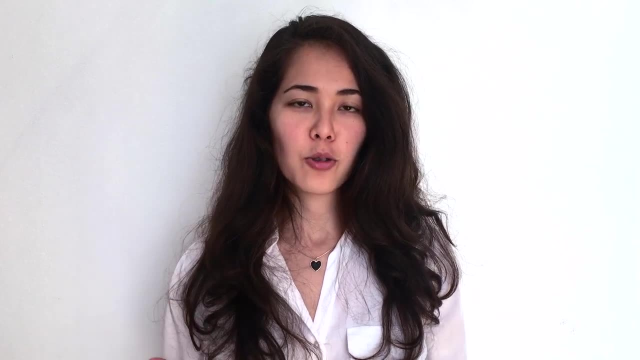 found a PDF somewhere. I downloaded it on my Kindle and I struggled a lot because it was difficult to read it in the small space, because when they explain something it's not just one sentence. Each topic that you want to understand in aerospace it could take from three pages and up, But the textbook 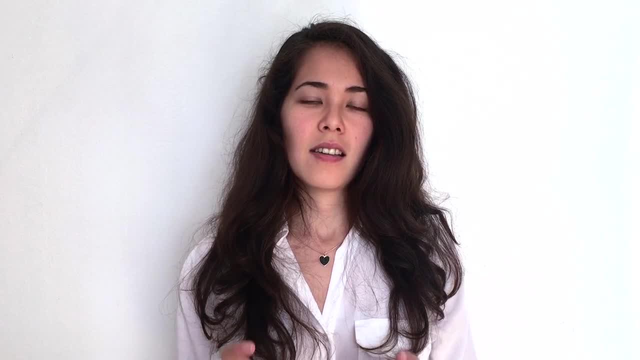 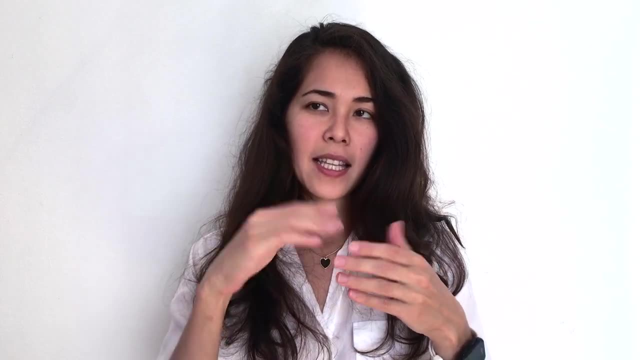 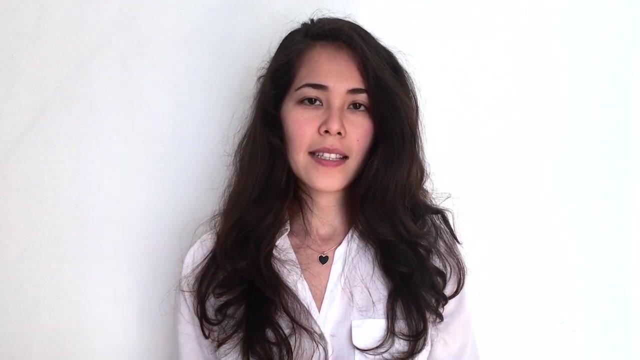 itself was interesting, but very condensed because it was very thin. they explained the material very, very fast so they didn't explain the middle steps between calculations or between explanations. so it was a textbook that takes long time to read because you need, because after every sentence you need to. 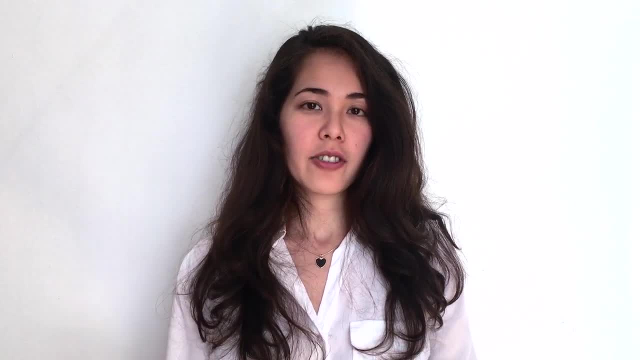 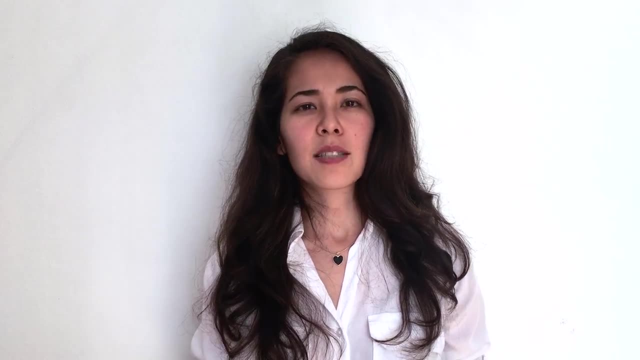 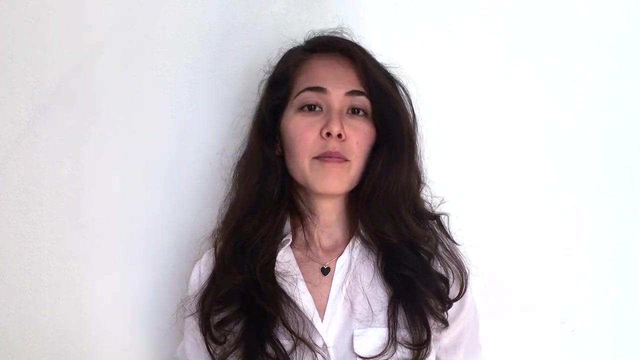 understand how to get to the next sentence, but if you're interested in electric propulsion, this is a textbook that I recommend. all right, so those are all the textbooks that I remember from my college years and the ones that I wanted to recommend to you guys, but the ones that I liked the most were the 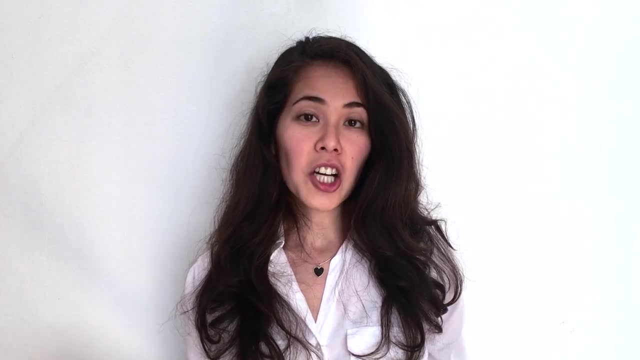 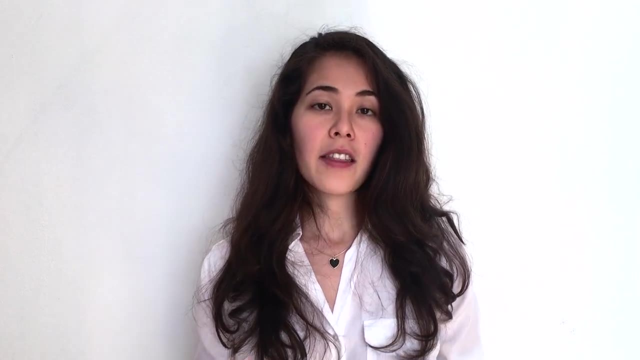 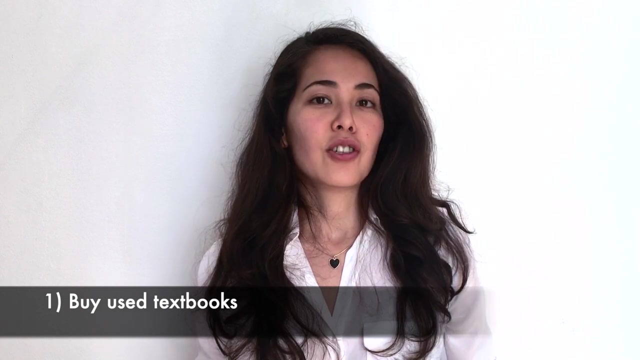 first two textbooks, all right, so now let's talk about how to hack the system and get your textbooks cheaper. so the first option that the university actual recommends you is the one that I recommend to you- is to go to the bookstore and buy used textbooks. you can also find used 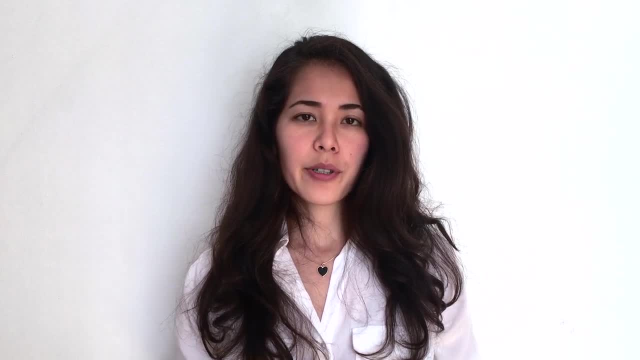 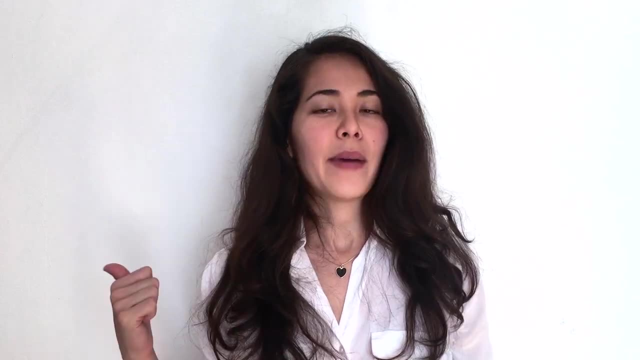 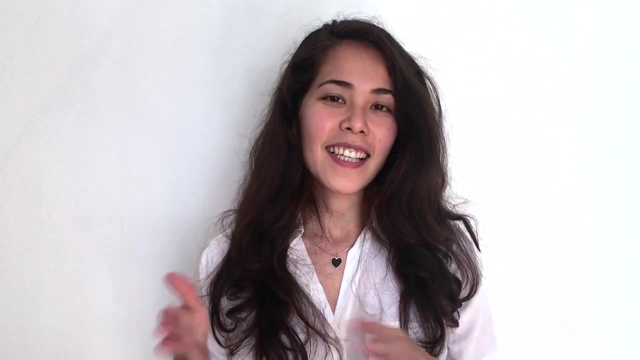 textbooks on Amazon and they are much cheaper than new textbooks. for example, when I bought a textbook for 60 bucks, I went back to return it and they only gave me $20 for it, so it's not a good deal. and then they sell it again as used. 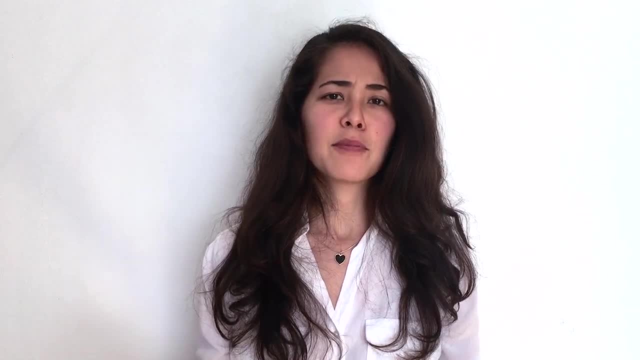 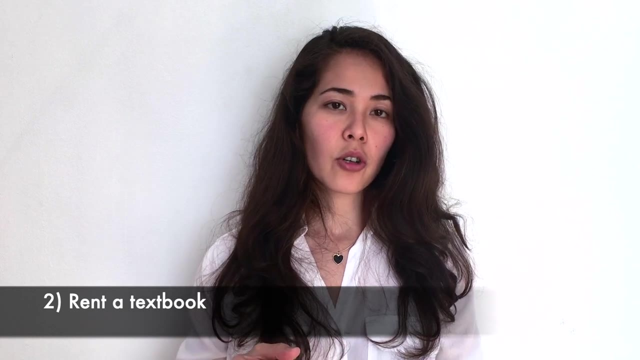 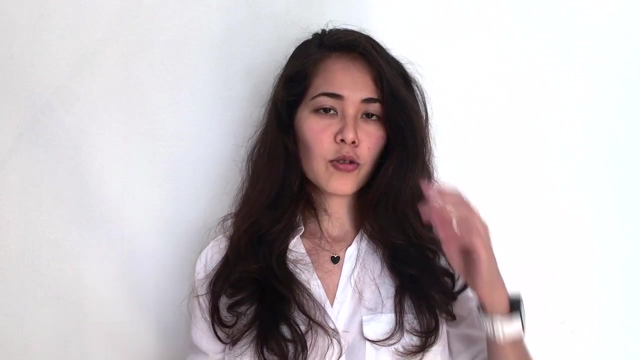 textbook maybe for $50, so used textbooks are not a good option to get textbooks. the second option: it is also from the bookstore, but you rent it and many online platforms can also let you rent the textbook for a year. but again, I don't think it's much cheaper. but 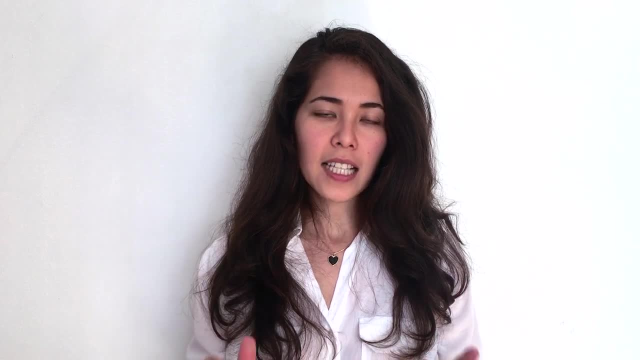 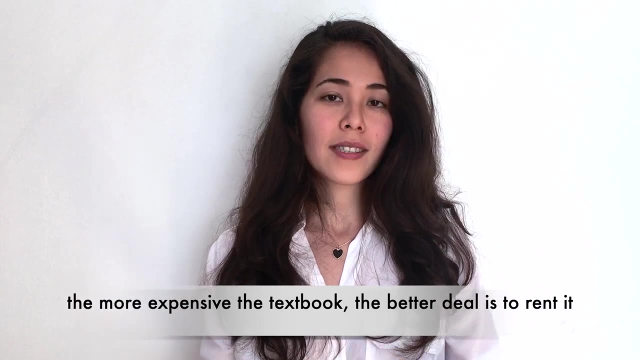 sometimes it is worth it. for example, if the textbook costs $200, you can rent it maybe for $90 per year. so you save a lot of money and you can rent it for a year. so the third option is the method I highly recommend because I used it. 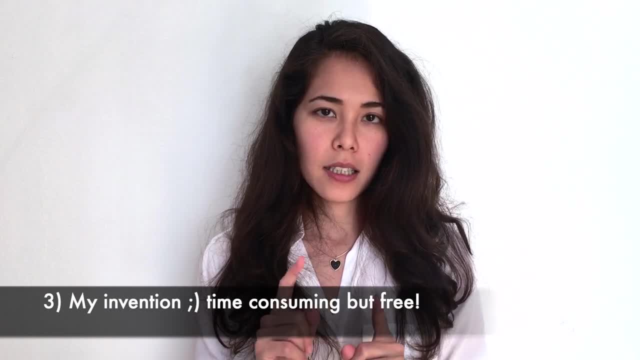 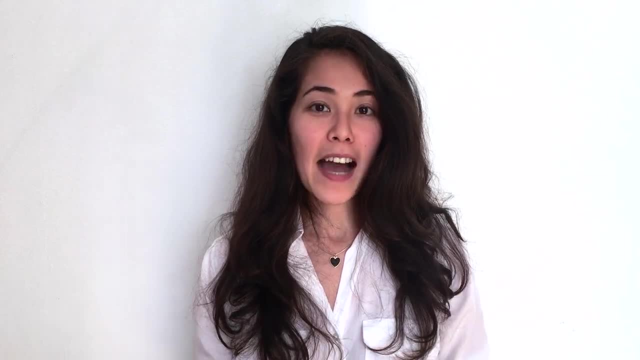 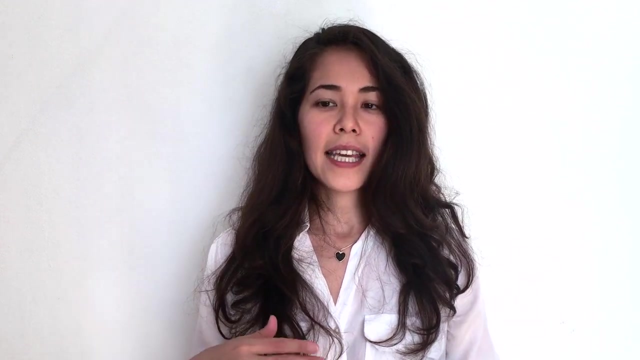 myself, and it's also time-consuming, but it's free. so you go to the library at the University find this textbook that you need for your class. usually they have them available, but you can only take it from the library for one day or something like that, maybe two hours, I don't remember. but you can take it for. 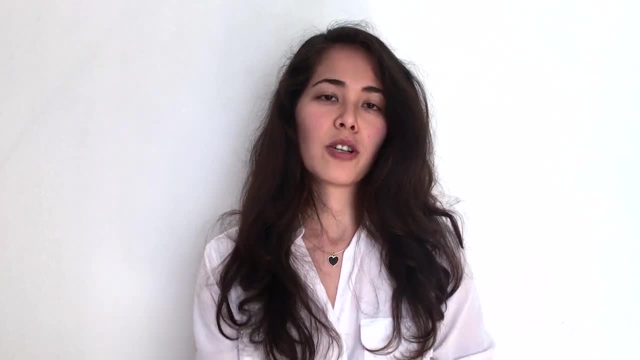 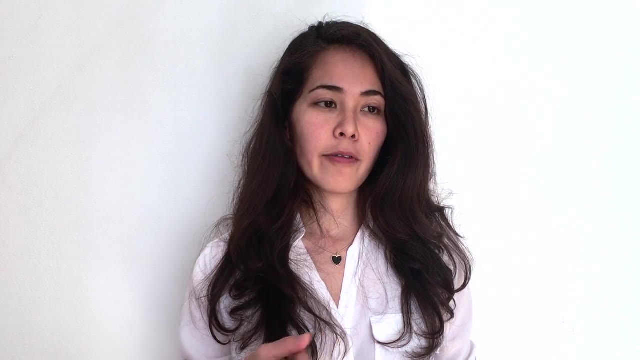 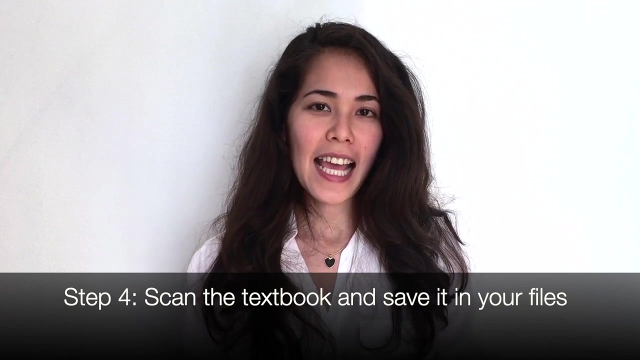 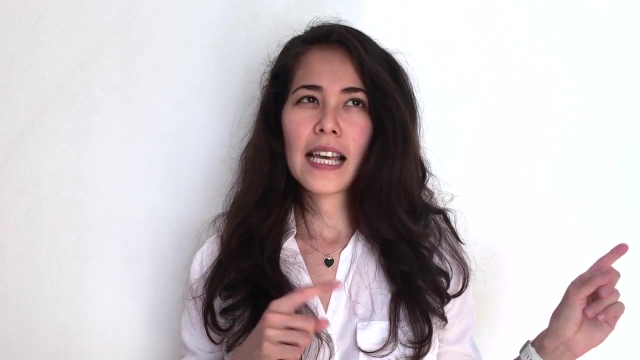 the whole semester because they don't have textbooks for everyone. so that's not an option to take it for one year. so basically you go to a library, get that textbook for two hours, then find a scanner, then scan the textbook, save it as PDF and save it on your USB Drive or whenever, maybe in the cloud, because in 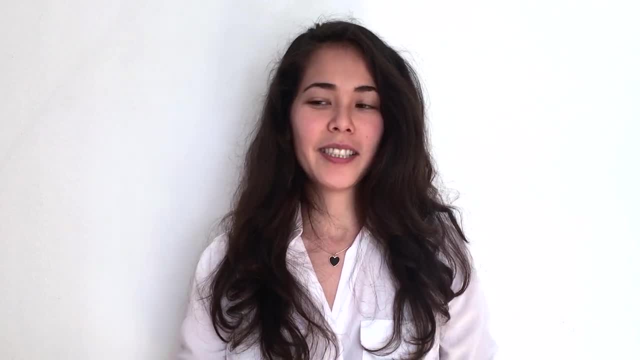 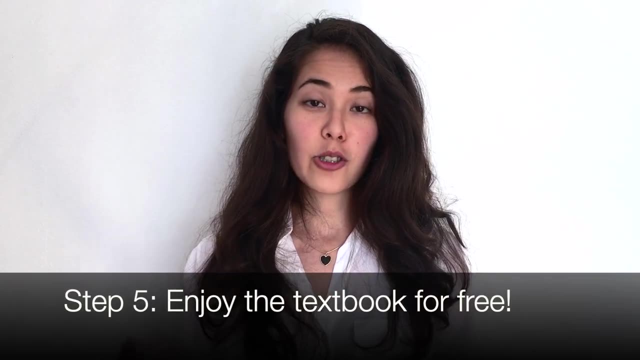 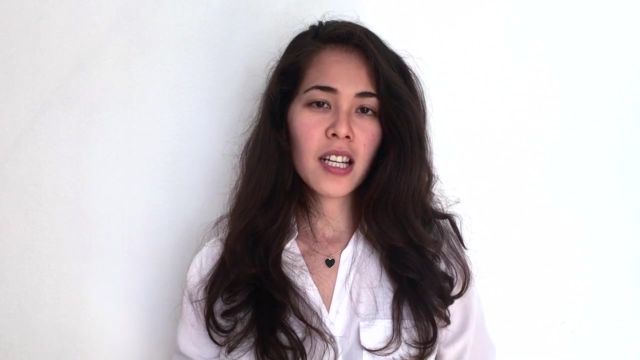 my time the cloud was not that popular. it did not have a lot of space. I only had like five gigabytes in Dropbox. so then you use your scan for free, because usually they have scanners in the library provided for free. so that's the method I used for some of my classes and obviously it's a lot of work. 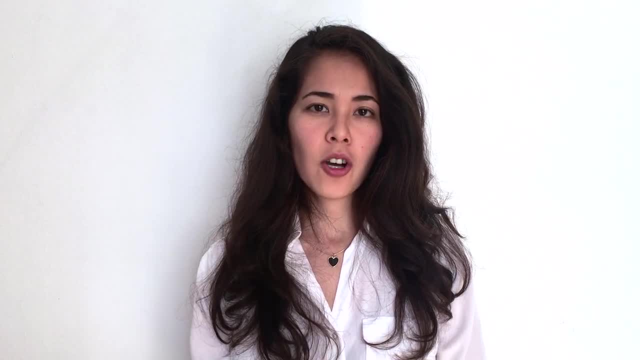 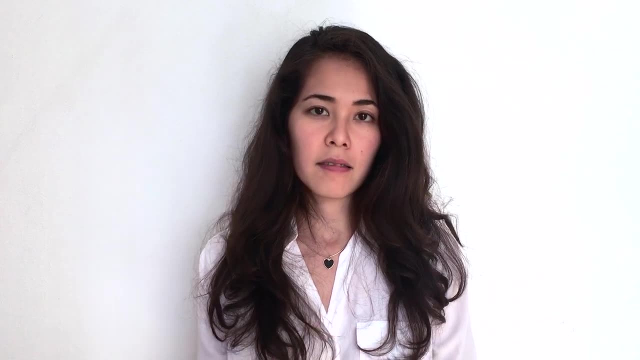 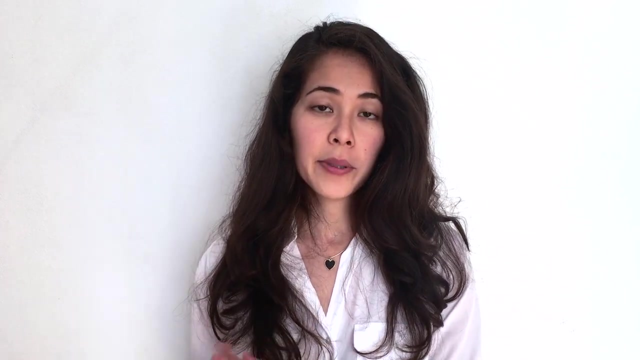 and a lot of time to scan a thick textbook. but what you can do is scan by chapters. for example, for the first two weeks just scan five chapters and use it as you go, and then, when your professor goes to the next topic, just scan some more chapters, so that way you will not spend five hours. 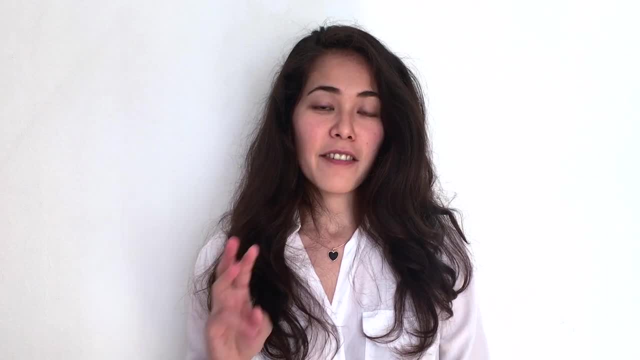 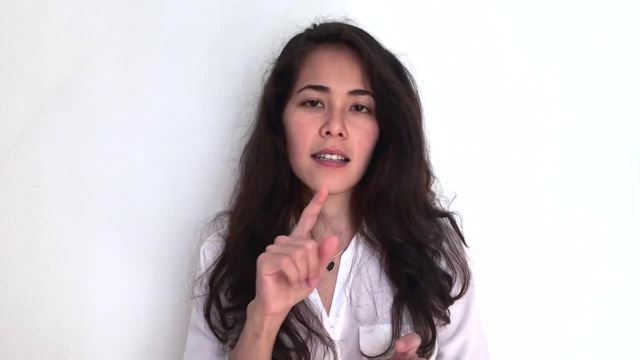 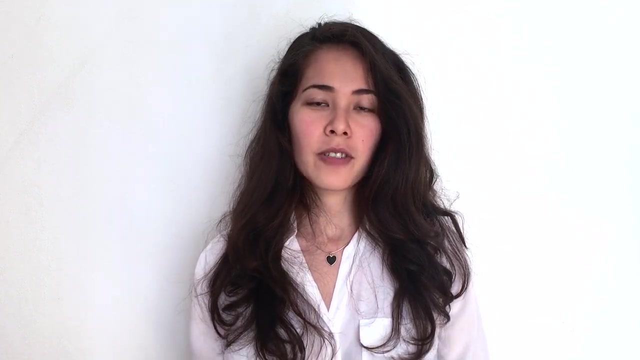 one day to scan the whole textbook. and the fourth option is very simple. you just go online and google the name of the textbook and add PDF or free, and then go through hundreds of pages trying to find a free version. but I didn't have enough time to do that, so I'm going to show you how to do that in the next video.